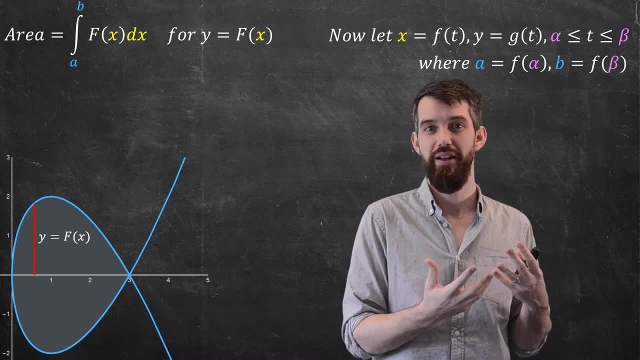 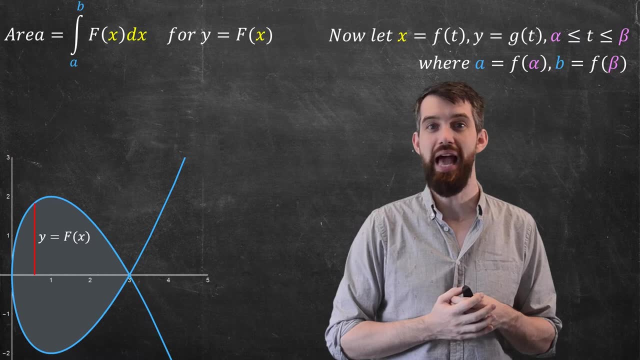 values, that t is constrained between an alpha and a beta. You can line them up with the previous formula by saying that the a is the f. Remember, f is the function that represents the x at the value of alpha and the b is equal to the f at the value of beta. But nonetheless I have to switch. 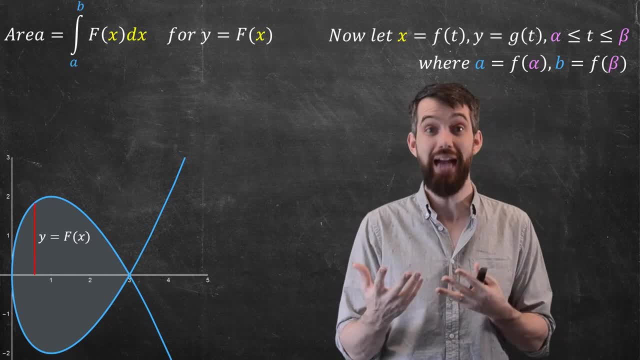 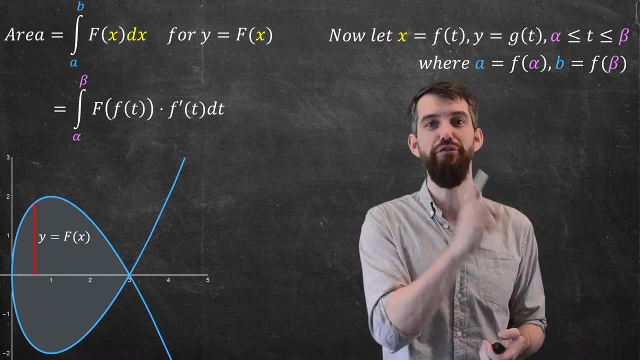 from a's to b's, to alpha's, to beta's, to keep the difference between x and t separate. And then, if I want to plug this in, I'm going to claim I get the following formula: I claim it's an integral from alpha to beta, It's an integral with respect to t. It's got a dt there And then it's big f of. 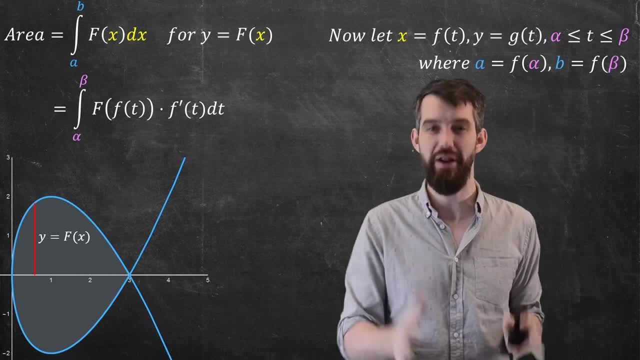 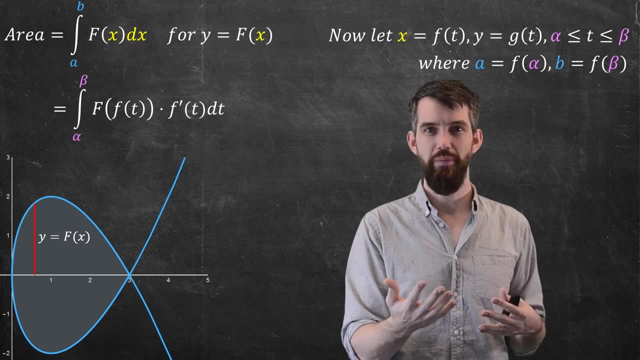 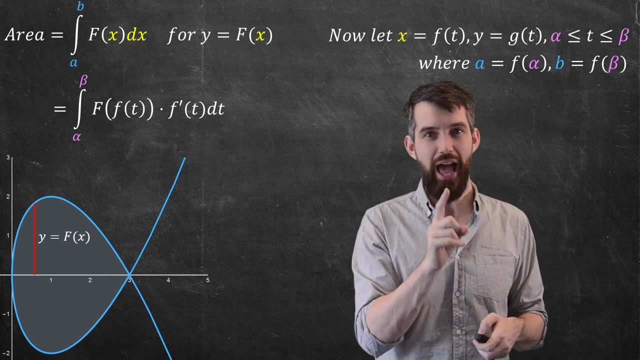 little f times f prime. Okay, why do I write this down? Well, this is a substitution rule. Recall how typically substitutions we do a u substitution, But because I'm going between x and t's, I'm going to do an x substitution here. That is, if I look at what f of t is, f of t, the lowercase f of t, is nothing but x, And then 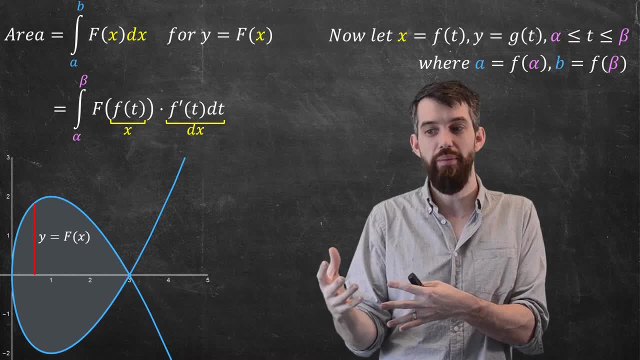 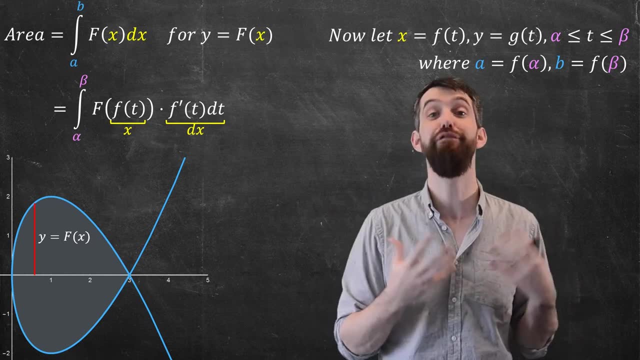 if I look at what f prime of t dt is, well that's going to be the same thing as dx. So if you apply the substitution rule to the second formula, you get precisely the first formula. It's just. I'm not doing a u substitution, I'm doing a sort of x substitution, Just a change of the order. 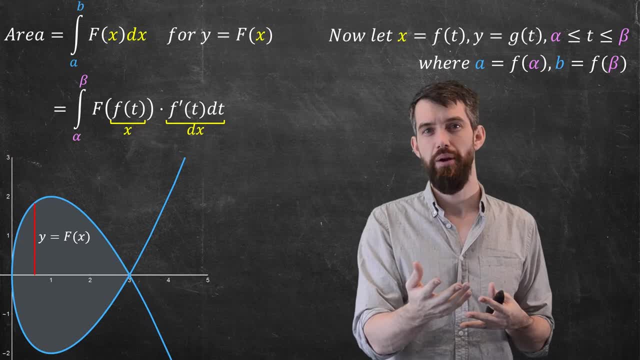 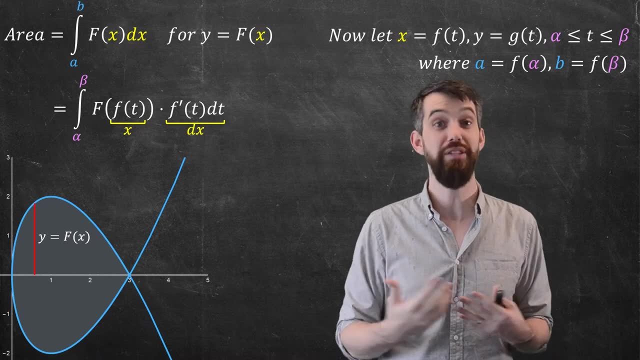 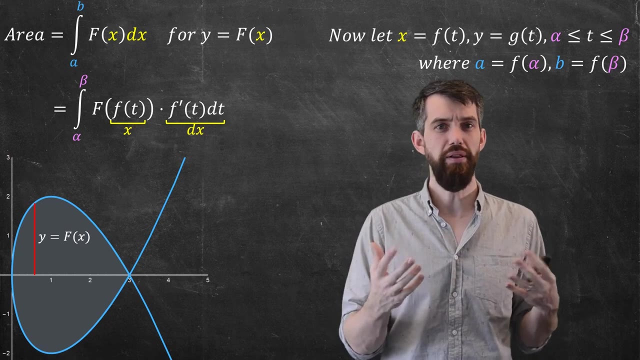 By labeling, But nonetheless the same idea. All right. well now let me look at this capital f of lowercase, of f, of t. Remember, capital f is representing the y, It's representing the height And because it's a composition, the innermost thing is a function of t. But this is 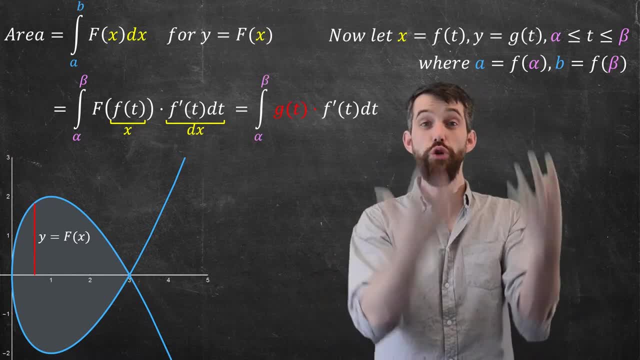 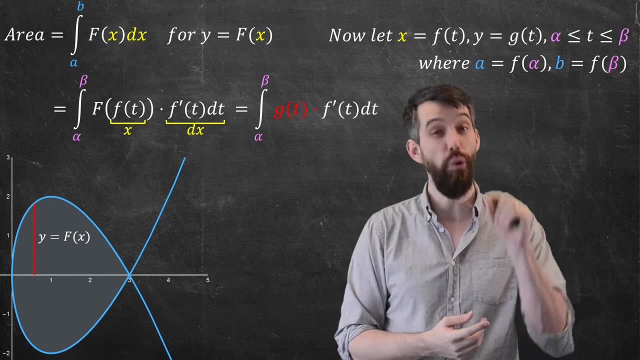 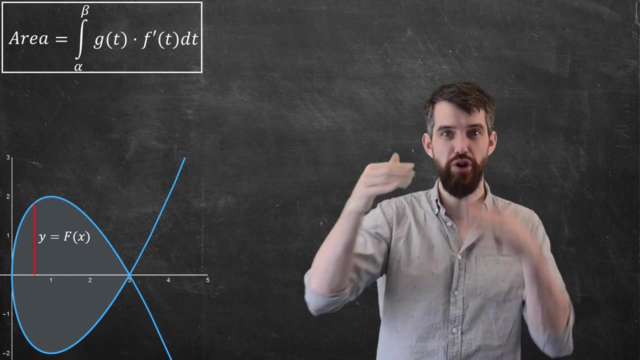 nothing but the function g of t. g of t also represents y, Represents the height above the x-axis, And it's also a function of t. These are the same thing. So capital f of lowercase of f of t, nothing but g of t. All right, so that's my formula for the area beneath some parametric. 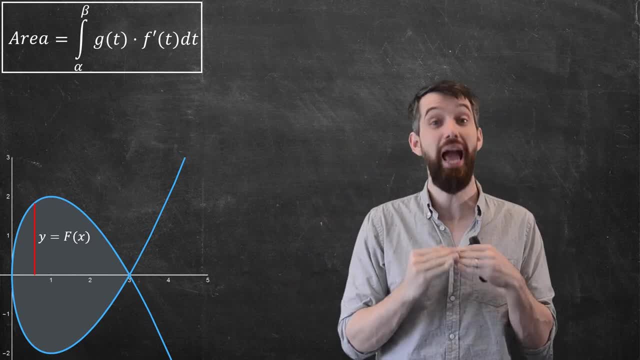 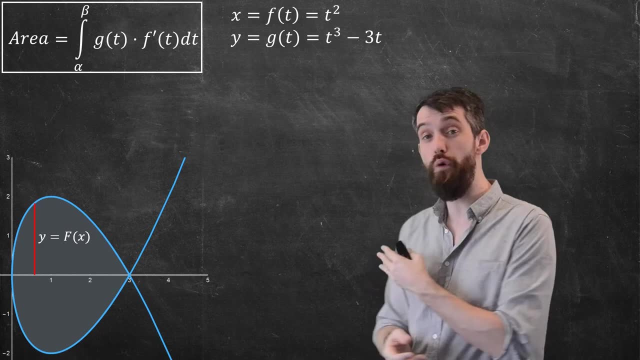 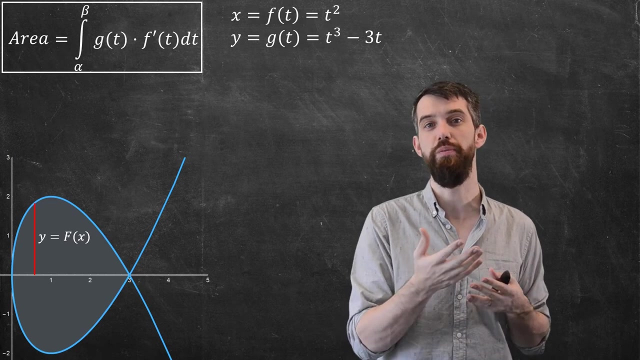 curve down to the x-axis and in between the endpoints of t equal to alpha and t equal to beta. All right, so let's do that for the specific example we've seen before. In this example, the x or the f of t was t squared and the y or the g of t was t cubed minus 3t. I'm going to have to. 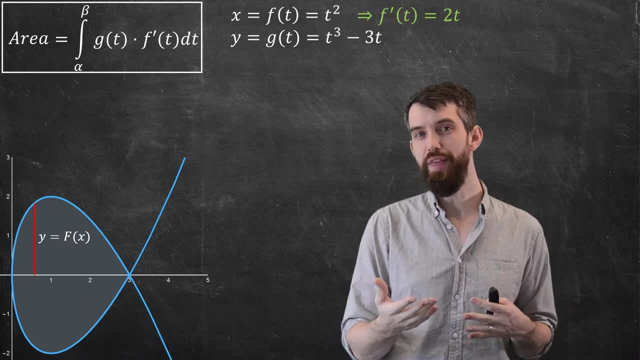 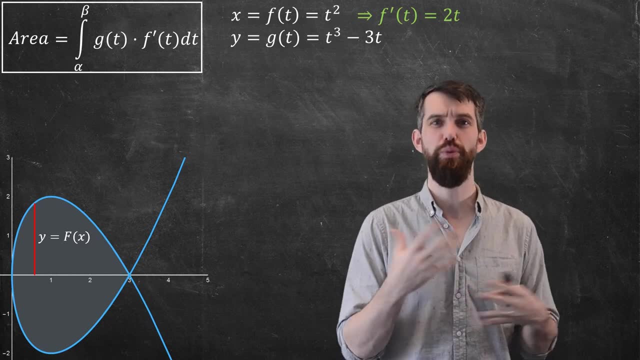 compute f prime so I can go and do that f prime is 2t. And then I want to figure out the endpoints for my integration. Now I'm going to do one little trick, which is to exploit some symmetry. I'm only going to consider the top half of this. that allows me to do the stuff above the. 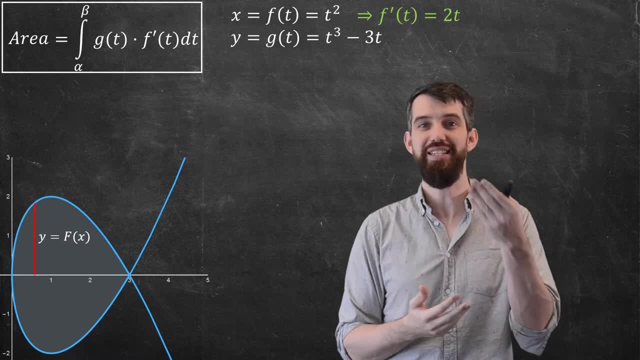 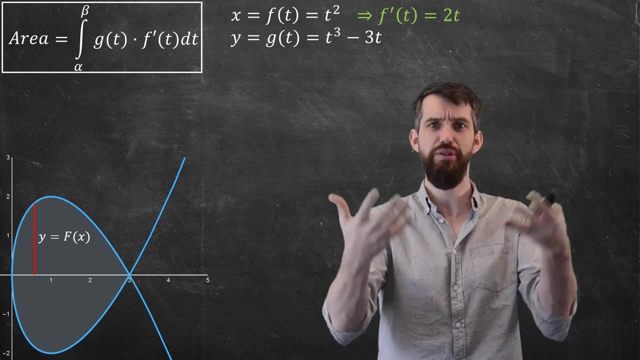 x-axis, and then I can multiply by 2.. Indeed, for any fixed x value, the y has got a positive and a negative. It's completely symmetric over the x-axis. So I'm allowed to do this. Just consider the top half and multiply by 2. trick Well, what are the endpoints for just the top half of this? 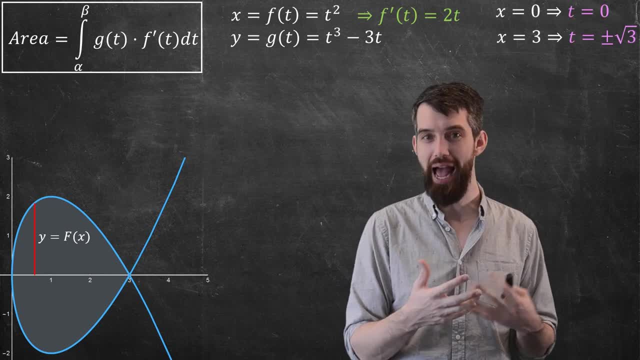 Well, if I plug in x to the top half of this, I'm going to get x to the top half of this. This is sort of the left endpoint in x. Plugging in x equal to 0 gives me that t is equal to 0. So 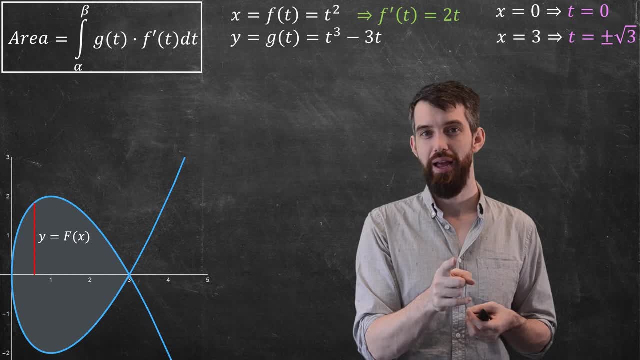 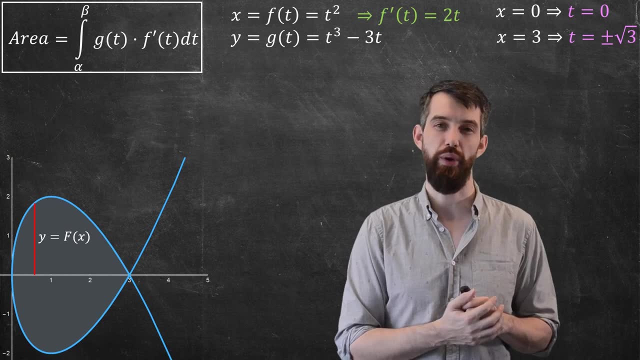 when t is 0, I'm at that leftmost point, And then when x is equal to 3, I get that t is either equal to plus or minus, the square root of 3.. Now it's correct that there's two different t values here. 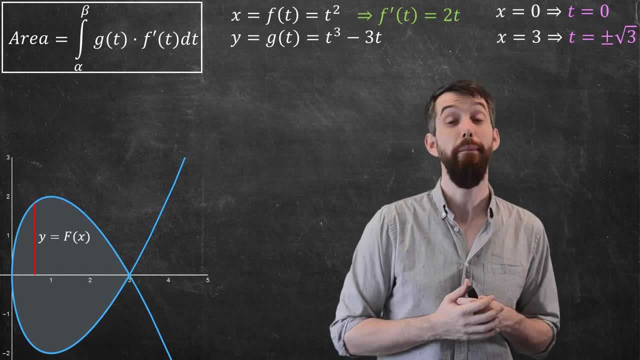 because, for example, if you started at 3, 0, say at t equal to minus root 3, and then you can carry on increasing your values of t until you get to t equal to root 3 and you've gone around the loop, ended up exactly back at 3: 0.. 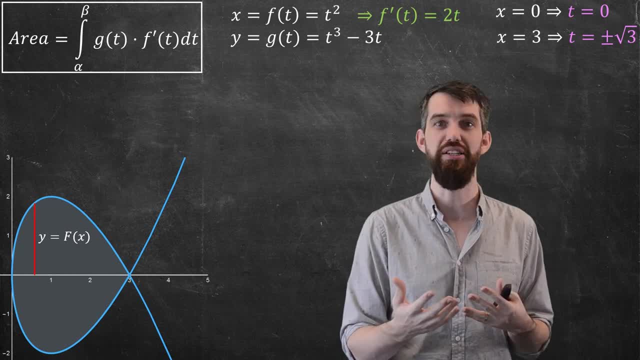 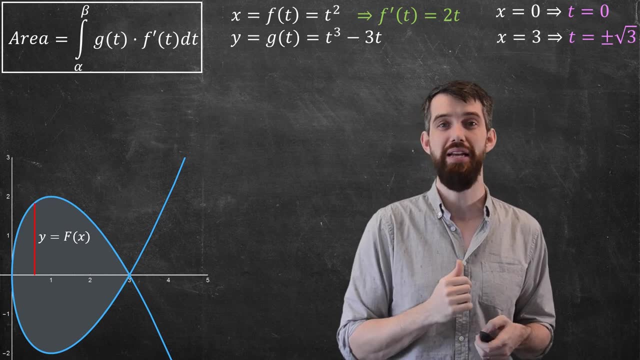 But because I'm only doing the top half, I only need to do it once. I'm going from the left to the right. I'm just going to use t, equal to the positive square root of 3 multiplied by 2, in my answer. So what do I have? I have that 2 out the front because I'm just doing the top half. Then 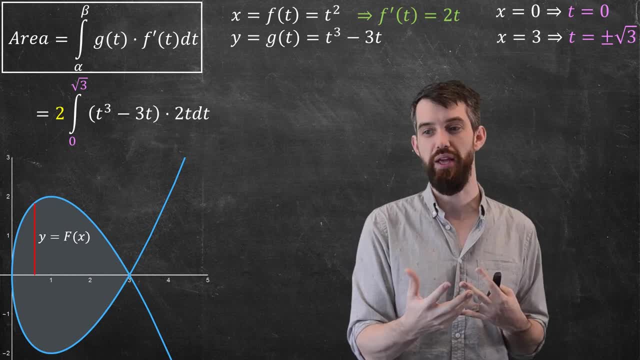 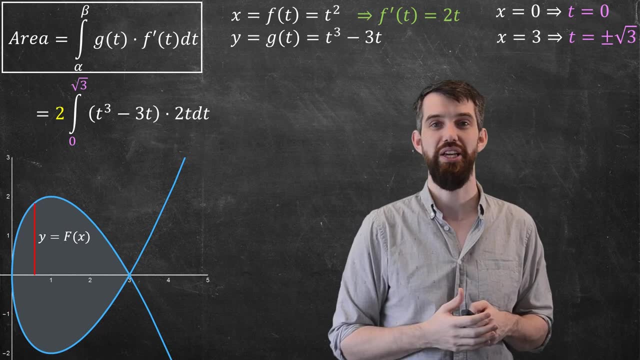 the integral from 0 up to positive square root of 3.. And then I put in my g of t and I multiply my g of t by my f prime of t, And well, this is just some particular integral. I can go off and compute. 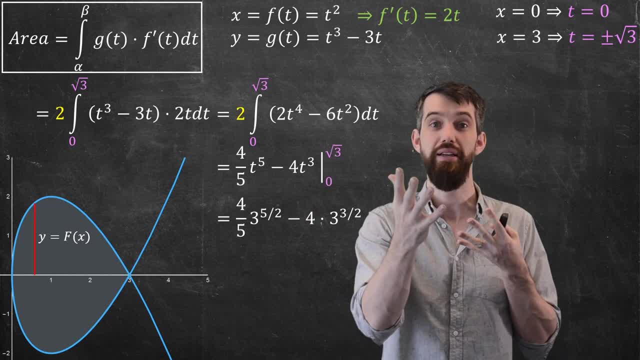 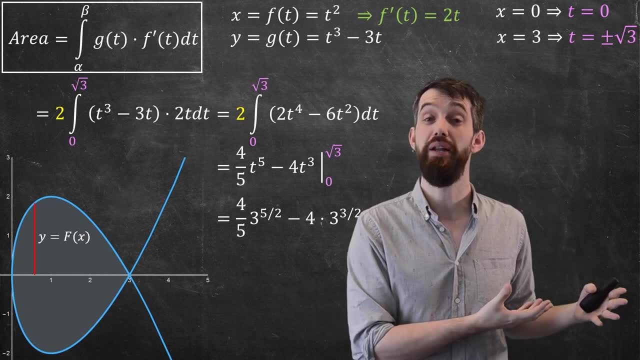 it and what do I get? Just whatever this thing is, It doesn't really matter, So I'm just going to do it. It doesn't really matter, It's a definite integral. So now we have replaced our ability to do areas under curves not for y equal to f of x, but for parametric functions. By the way, I'll note that. 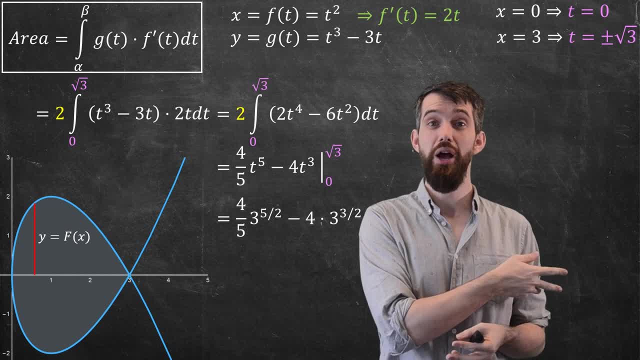 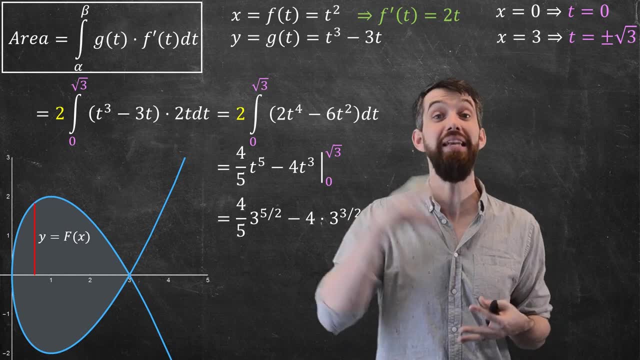 I'm doing a simple example here, but if you recall, back when you had calculus 1, we had issues, for example, where a function was above and below the axis and you had to break it up into two regions and the portions beneath the axis were going to count negatively and the portions above would.